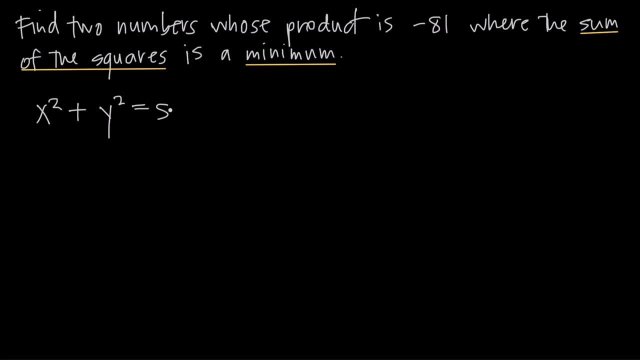 ahead and call the sum of the squares. here s. So we have s. the sum of the squares is equal to x squared plus y squared, So we want to try to minimize s. Now, once you have a function for whatever you're trying to maximize or minimize, the next thing you need to do is make sure that. 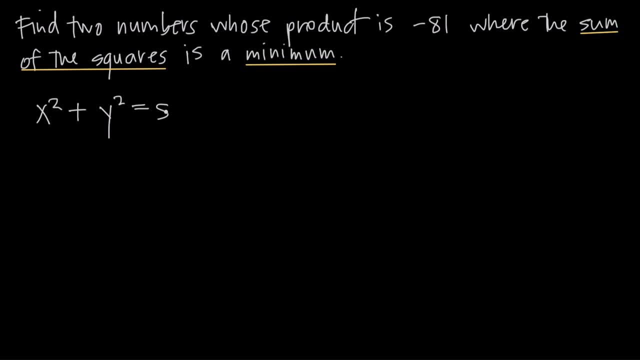 it's in terms of only one variable. Well, right now s is in terms of both x and y, two different variables. So we need to get it in terms of one variable. and that's where we go back to the original problem, because we've been told that the two numbers have a product of negative 81. So we 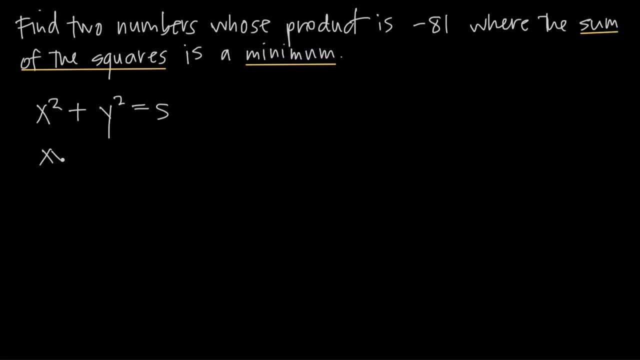 can write a second equation. Remember, our numbers are x and y. So x times y, their product, when we multiply them together, is going to be equal to negative 81.. So now, if we go ahead and solve for one of these variables, 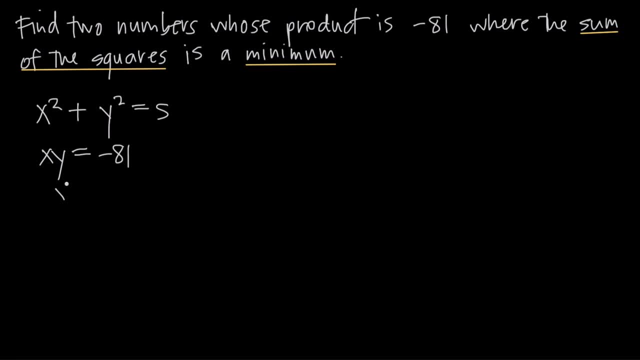 let's go ahead and solve for y by dividing both sides by x. we get: y is equal to negative 81 divided by x. Now we can take this value for y. So we have a value here for y and we have a value here y. So 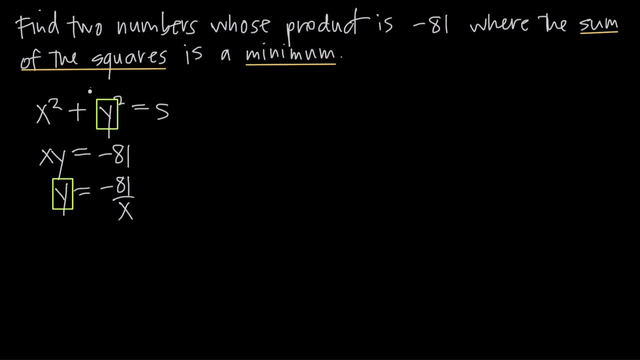 we can plug negative 81 over x into this equation for s, for y. So what we get then is: s is going to be equal to x squared plus instead of y squared, we'll get negative 81 over x squared. Now we want to simplify this as much as we can, So we're going to get s is. 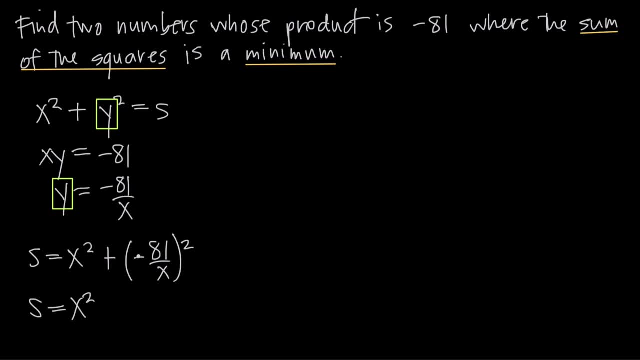 equal to x squared. When we square the negative sign, it's going to become a positive, So this negative will drop away. 81 squared is 6561.. When we square the x in the denominator, we're going to get x squared. Now, remember our steps. were we identified in the problem that we were asked to? 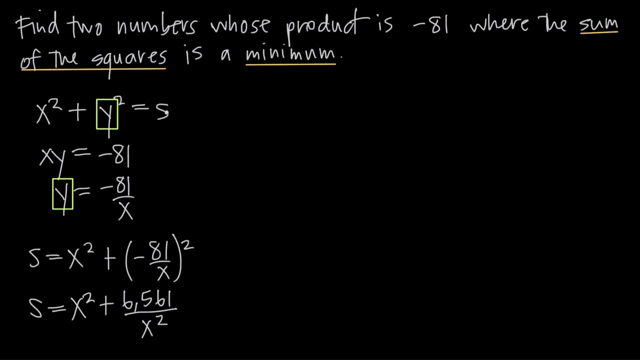 minimize the sum of the squares, which means we needed to generate a function for the sum of the squares. We did that, We got it in terms of one variable and we simplified it. So, now that it's simplified, and in terms of one variable only, our next step is always going to be to take the 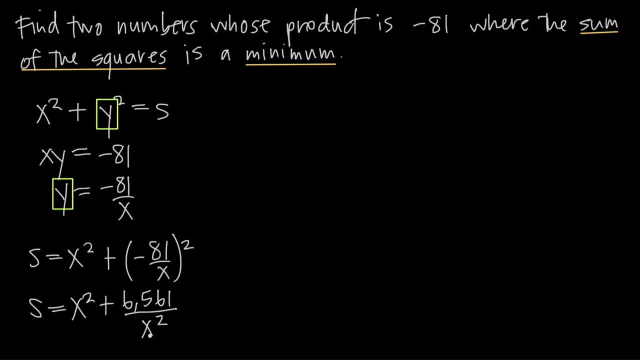 derivative of this function. First of all, before we take the derivative, let's go ahead and move this x squared in the denominator into the numerator. Remember, this is a rule of exponents. We're going to get: s is equal to x squared plus 6561, x to the negative 2. We bring this x squared. 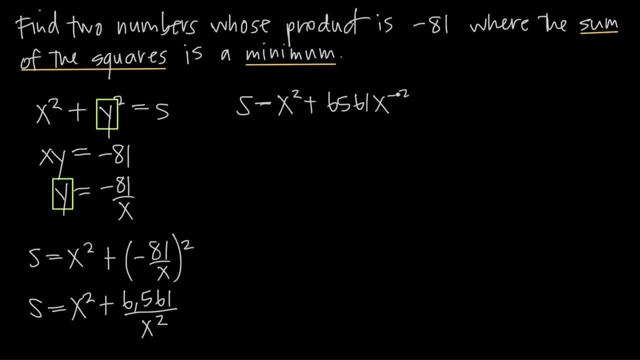 into the numerator And the exponent changes from a positive to a negative. So now we have our function s, We need to take its derivative. So the derivative we'll call s prime, And when we take the derivative we're going to get 2x, 6561 times a negative. 2 is going to be a negative, 13122 x. And then power rule, we subtract. 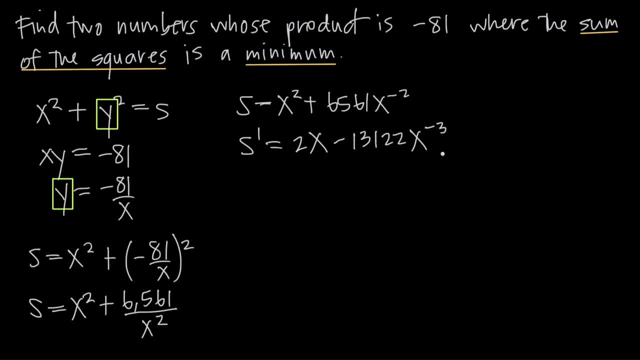 1 from the exponent negative. 2 minus 1 is a negative 3.. Now, if we rewrite this in terms of positive exponents, we're going to get s. prime is equal to 2x minus 2x squared, So we're going to get the. 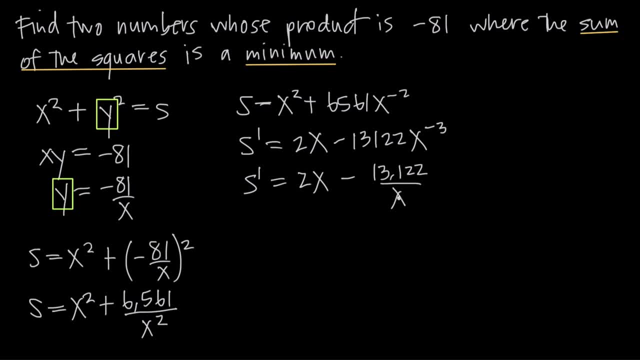 derivative minus 13122 over x cubed, We move the x to the negative. 3 back to the denominator. The exponent changes from a negative to a positive. Now, once we have the function for the derivative, what we always want to do is set this equal to 0, so we can solve for the critical points of the 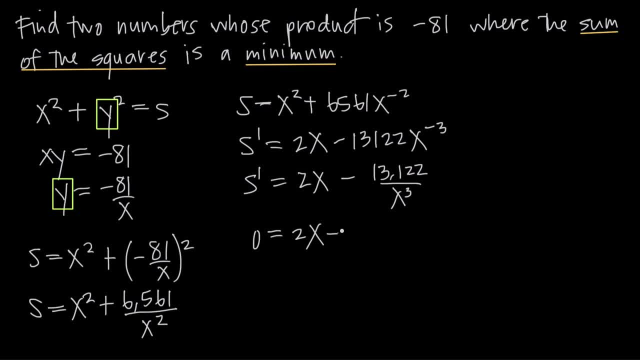 function. So we'll set s prime equal to 0 and we'll get 0 equals 2x minus 13122 over x cubed. Now we want to solve for x, And what we'll do is we'll add 13122 over x cubed to both sides. We'll get 13122 over. 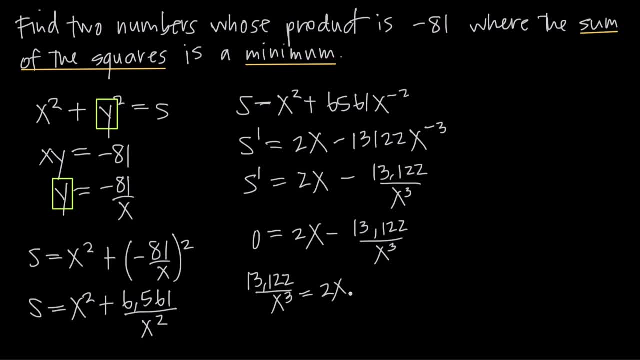 x cubed is equal to 2x. When we multiply both sides by x- cubed, we get 13122 is equal to 2, x to the fourth. When we divide both sides by 2, we get 6561 is equal to x to the fourth. And when we take the fourth root of 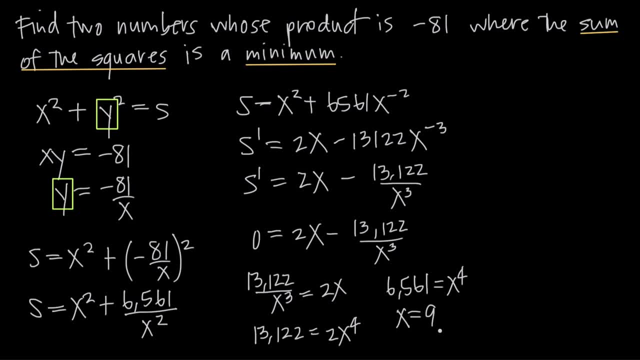 both sides to solve for x, we get x is equal to 9, because 9 times 9 times 9 times times 9, or 9 to the fourth, is equal to 6561.. So we have this value for x, but we're not done. 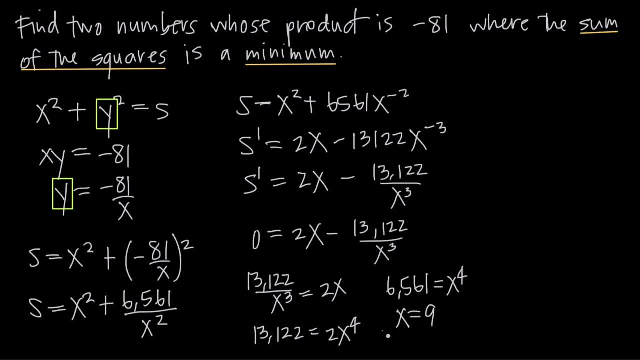 We need to make sure this is a potential critical point of the function. We need to make sure it is in fact a critical point. not only that it's a critical point, but also that it minimizes the sum of the squares. 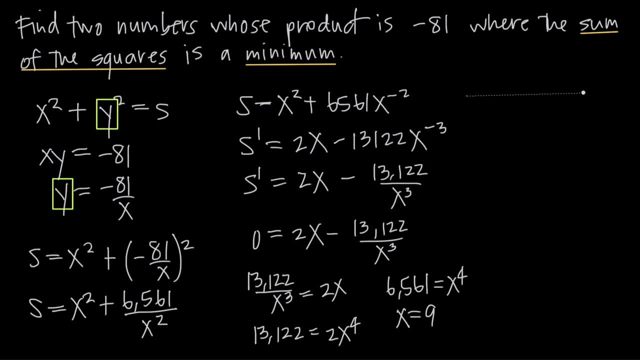 So what we want to do is go ahead and draw a number line. This is going to be our first derivative test, And we call it the first derivative test because we're going to be testing the critical point in the first derivative. The first derivative is s prime, so I always 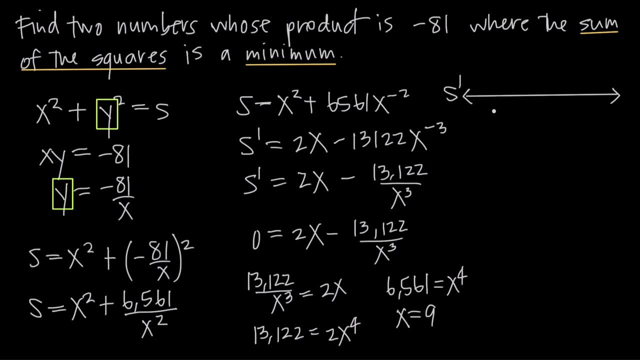 like to go ahead and say s prime next to my number line, to remind myself that I'm going to be testing this critical point in s prime. I want to go ahead and plot: x equals 9 right in the middle of the number line, so x equals 9.. 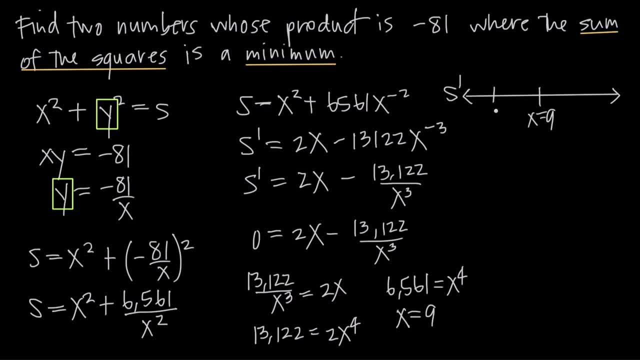 And then I want values on both sides of x equals 9.. So we'll go ahead and say: over here x equals 8, and over here x equals 10.. And these values- 8 and 10- on either side of the critical point, are the values. 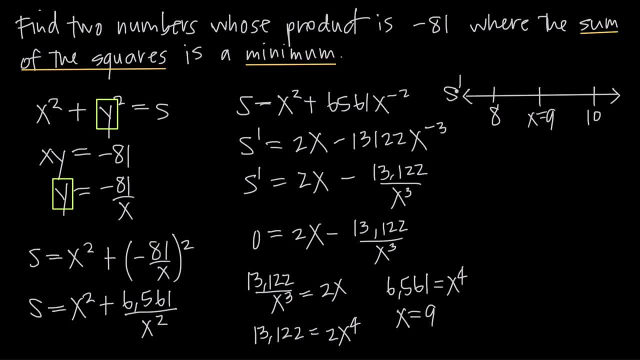 that I'm going to be plugging into my derivative s prime As part of my first derivative test. So if I say s prime of the value on the left 8, I'm going to go ahead and plug that in And I'm going to get 2 times 8 minus 13,122, all over 8 cubed. 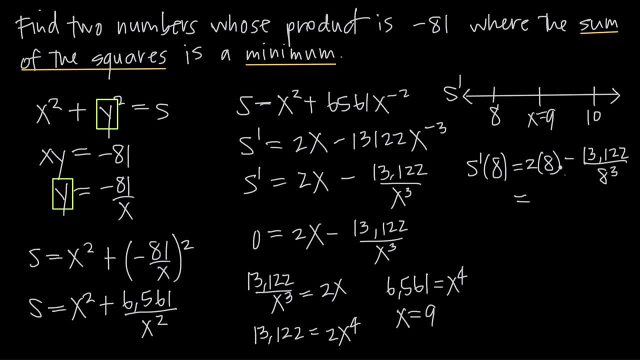 Now remember: what's important is not the exact value of this right-hand side, but whether the right-hand side is positive or negative. When I do this arithmetic here, what I see is that I'm going to get a value that's negative. 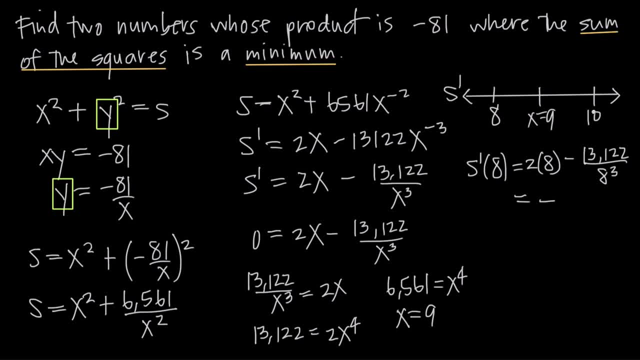 We'll come back to that in a second. I want to test the value on the other side, So I'm going to plug that into my first derivative And I'm going to get. s prime of 10 is equal to 2 times 10. 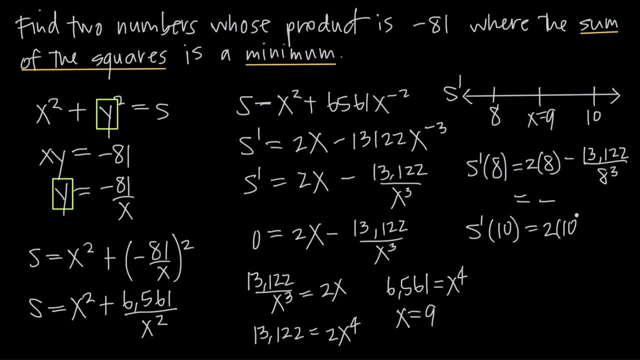 minus 13,122 over 10 cubed. And when I do the arithmetic on the right-hand side this time I get a positive value. So a negative value and a positive value. We want to go ahead and plot those on our number line. 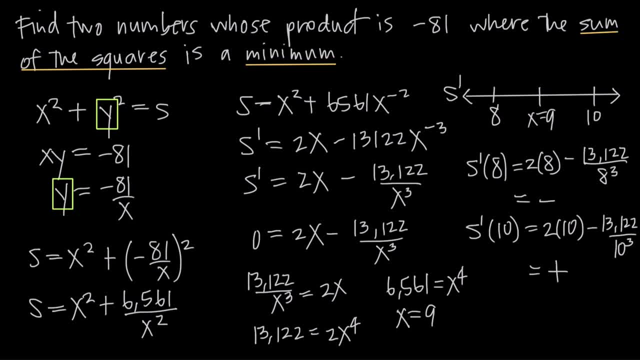 So because we got a negative value, what we can say is that the derivative is negative everywhere to the left of the critical point. So we're going to plug that in, And we're going to plug that in, And we're going to plug that in. 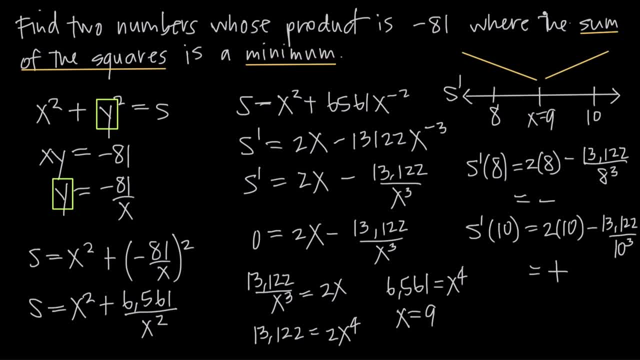 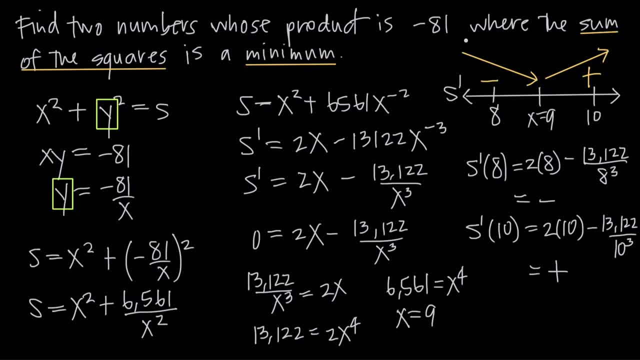 So when the derivative is negative, it means that the original function is decreasing. When the derivative is positive, it means that the original function is increasing. So we can say that to the left of x equals 9, the original function s, the sum of the squares, is decreasing. 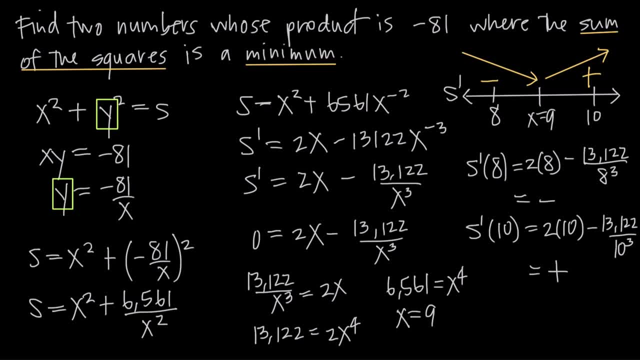 To the right of x equals 9, the sum of the squares is increasing, which means that we can see visually here that at x equals 9, that's the point at which the sum of the squares is minimized. So this is a critical point. It is the point that